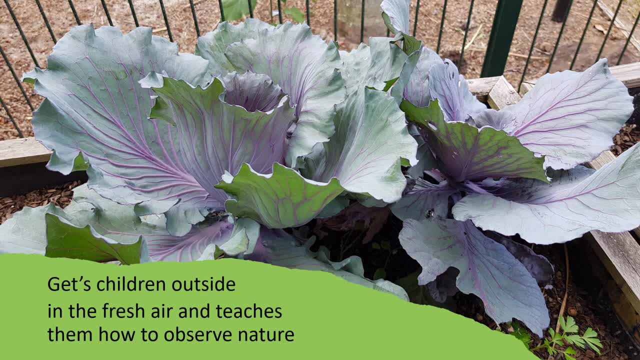 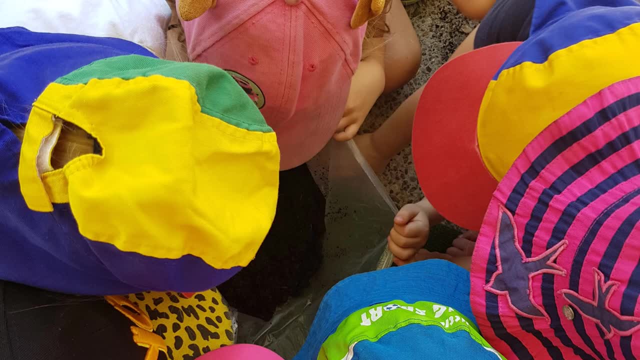 Observing nature is a skill that takes stillness and quiet, and this will be good for children. Cooperation As they follow the amazing growth stages of a new seedling and what they can do to help it thrive. children learn how to work individually and together as part of a team By participating in gardening. 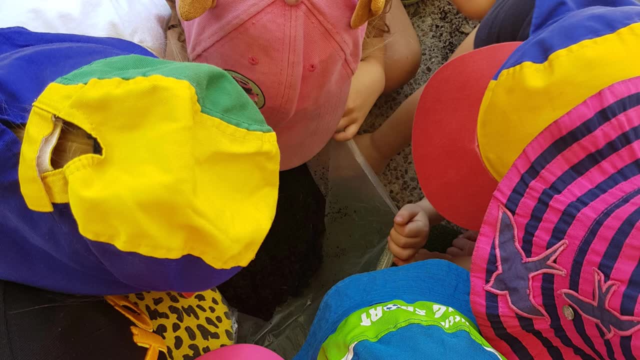 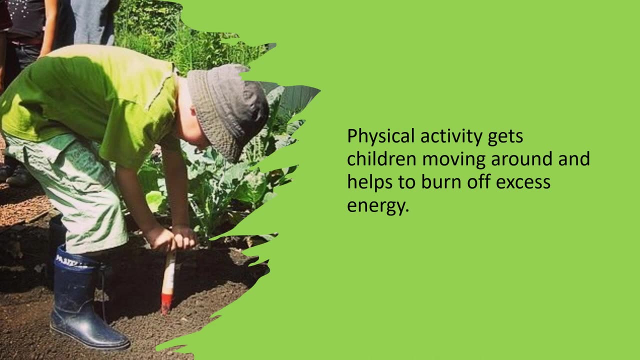 as a group, they will learn how to help you. Each other, share tools and teach others how to look after the crops. Physical activity- Gardening- is a fantastic adventure for children and gets them outside doing something fun and productive while spending time away from screens. As it is an activity that gets them moving around, they will be able to. 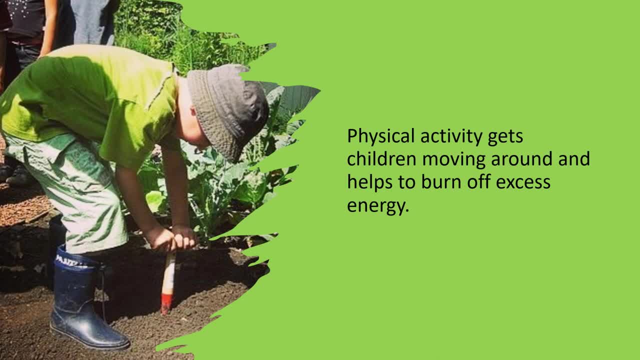 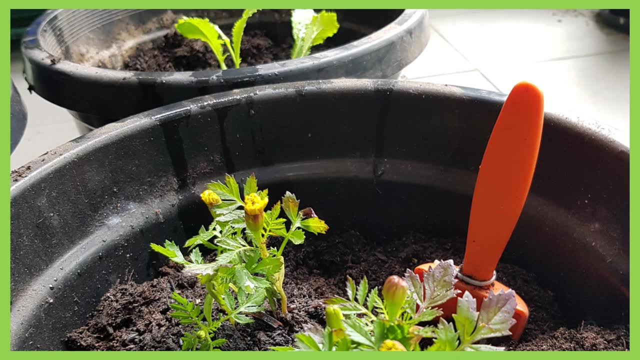 burn off any excess energy, so they will be better able to sit for a longer period when back in the classroom. As plants don't shoot up overnight, children will need to learn to be patient and wait for their flowers and vegetables to grow. This will reflect. 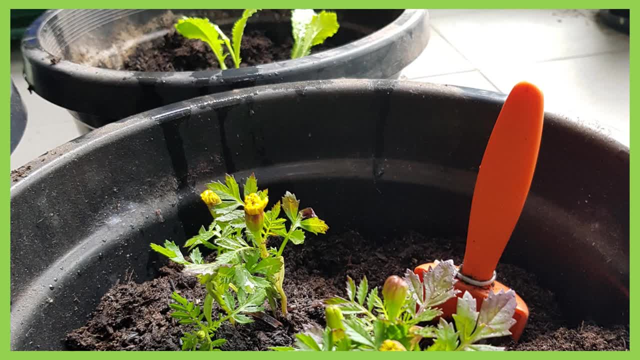 back in the classroom as they master this skill. They will also become more and more curious as they anticipate its growth. All in all, gardening is great for kids as it teaches them the lifetime skill of being able to grow their own food, and right now this is so important as the world becomes increasingly 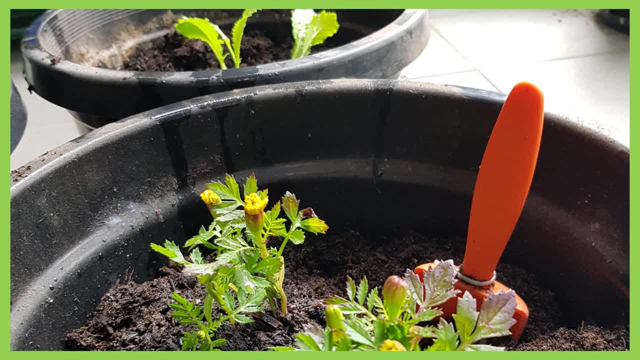 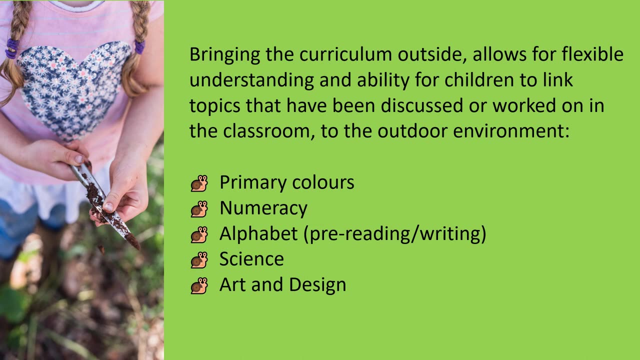 complex. giving them the tools to grow their own with the help of their parents, It will set them up for success in the future. As we go forward, the generations to come will benefit from having their own vegetable gardens in the family home. Link in topics By bringing the curriculum outside allows for flexible understanding. 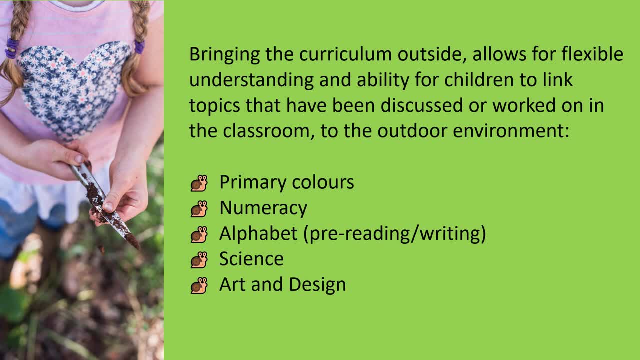 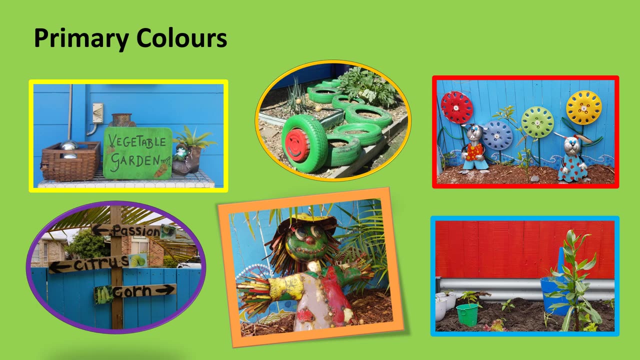 and ability for children to link topics that have been discussed or worked on in the classroom to the outdoor environment, such as primary colours, numeracy, alphabet, science, art and design. Primary colours: There is so much colour to be found in the garden. a whole activity can be based. 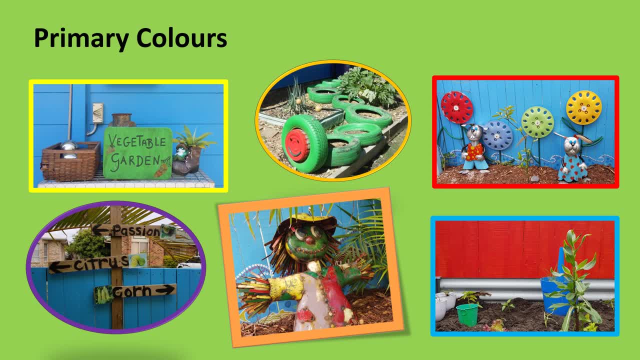 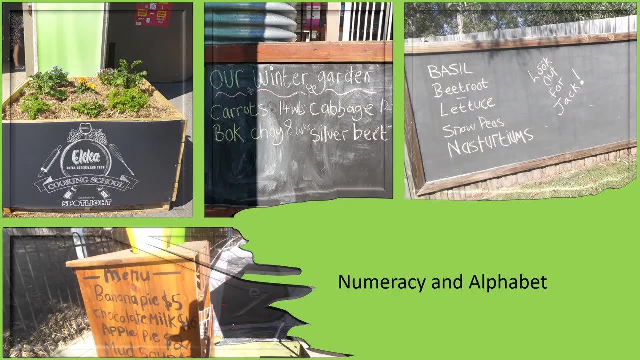 around the primary colours. Ask children questions such as what colour is the plant? or have them count how many flowers are red, yellow or orange? Painting the vegetable garden in bright colours makes it a more magical experience when they are outside. Numeracy and alphabet Writing labels for plants is a good way to practice. 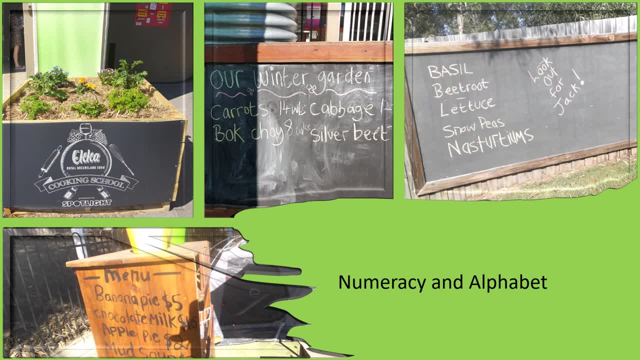 handwriting and you can try making signs out of wooden spoons that are stuck handled down in the soil and the cup of the spoon for writing on. Or take advantage of black balls for writing harvest times on as well. Ask children to count how many veggies are growing in the patch. You. 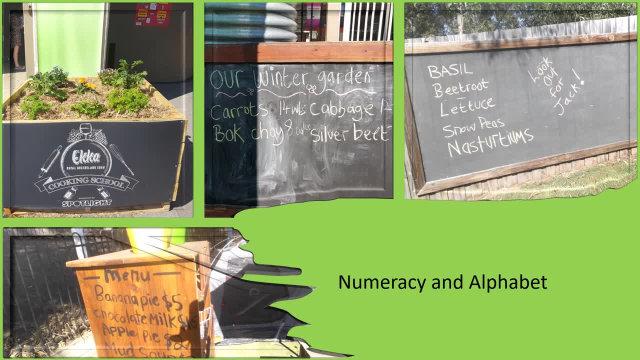 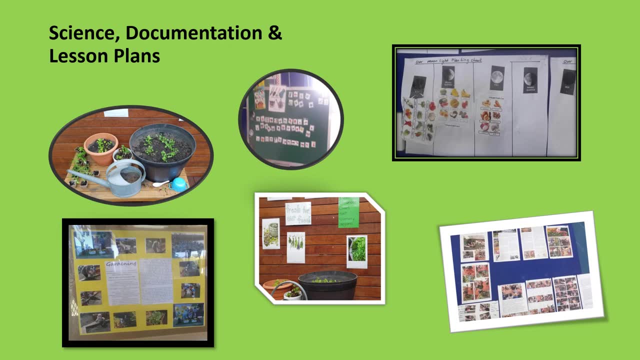 can create an activity where they add up the total of each vegetable growing in the garden. Science Gardening offers wonderful hands-on science lessons. Children can learn about biology, weather patterns, sunlight and plant growth. Learn about the super garden helpers using Wilbur the Worm Puppet, Live Worms and the Worm Farm or Camilla Caterpillar and Bella Butterfly. 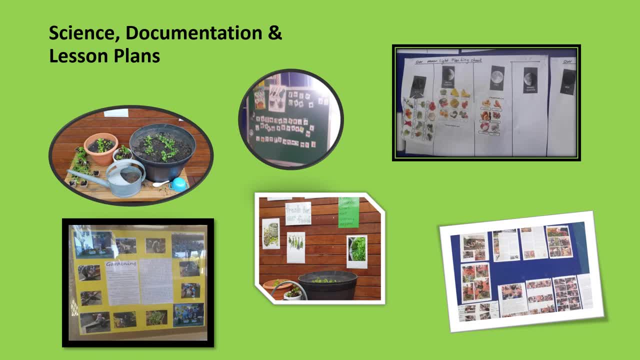 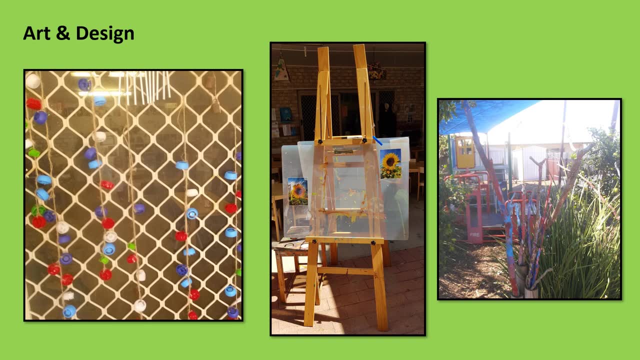 to observe the life cycle of a real-life butterfly. Art and design. The garden is a fantastic place for discovering art. It is everywhere in nature and children should be encouraged to get creative. They can paint colourful pots, stones or try setting up an. 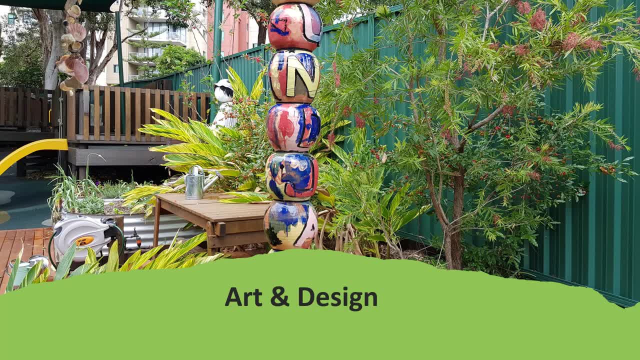 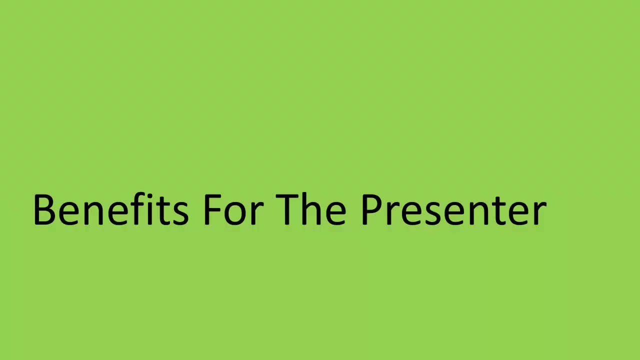 easel for painting flowers. You can even try making a totem pole for your garden. This one here is made from clay pots, but you can create an easier recycled version by using milk cartons and a broom. You will find this activity in this section of this course: Gardening and being around. 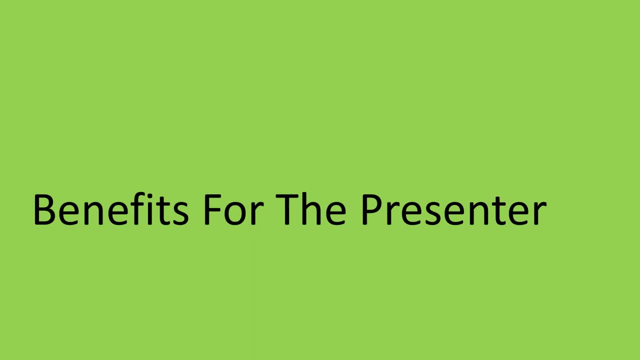 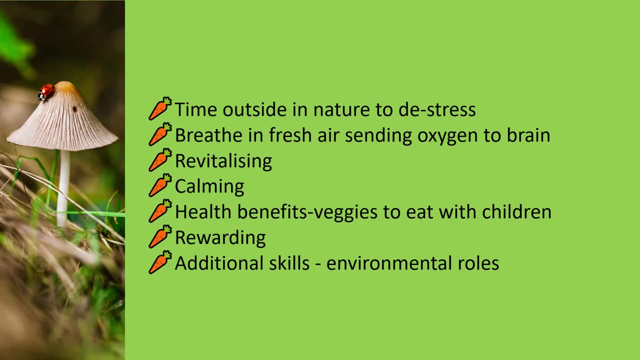 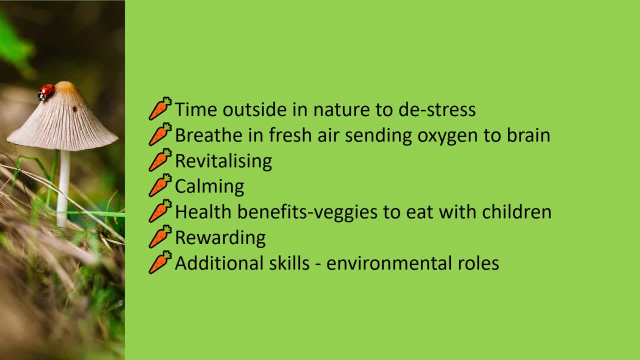 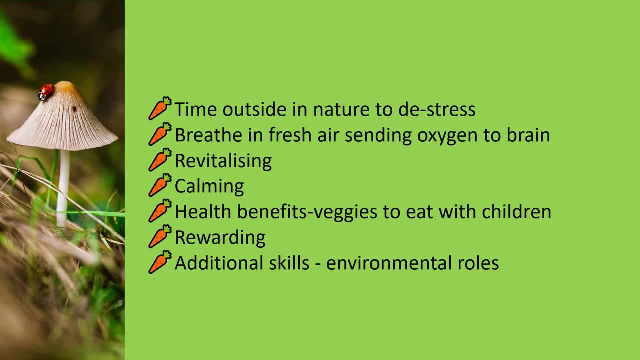 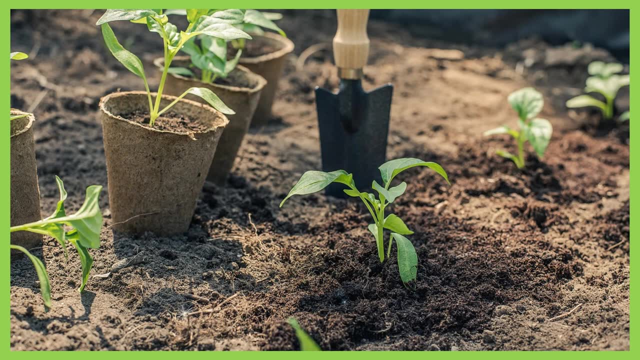 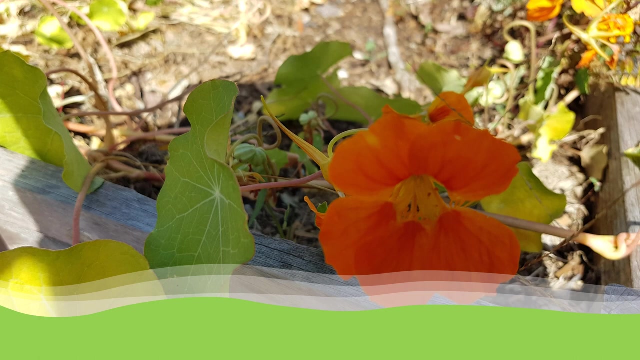 пом. Earth processing deodorants: Malone 1 stack 1але 2.5 Water Seaweed, maar Matt Wild. Sand Wild Earthing also helps with inflammation, improved sleep and improved blood circulation. Plant flowers in the patch. Not only do they attract the pollinators, but they are joyful and happy to be around. 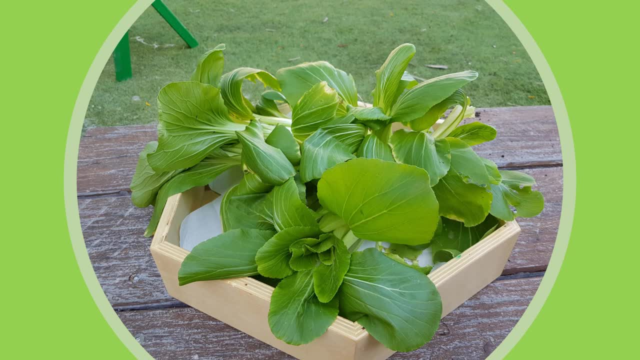 Another great benefit is being able to harvest and bring home crops that you can enjoy too, Improving your own health and nutrition whilst at the same time teaching children about healthy eating habits.